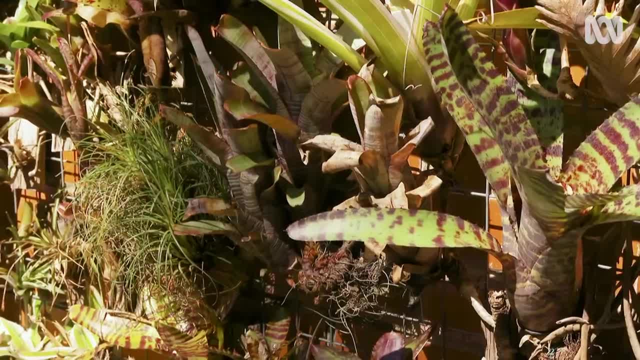 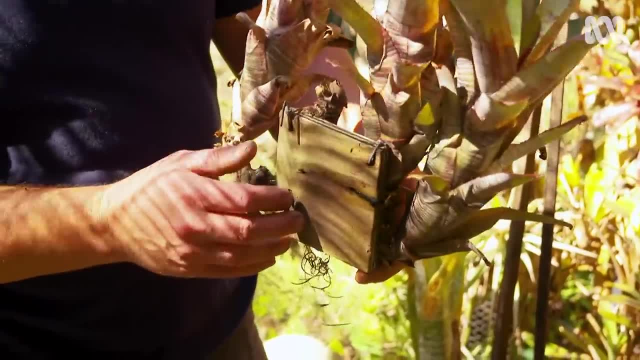 They just need their roots. They don't need their roots to attach to trees or to rocks. They can be mounted like a tree or they're mounted on timber. The timber's been connected so it's like a branch and they attach roots. So you've just got a couple of hooks on the back here. 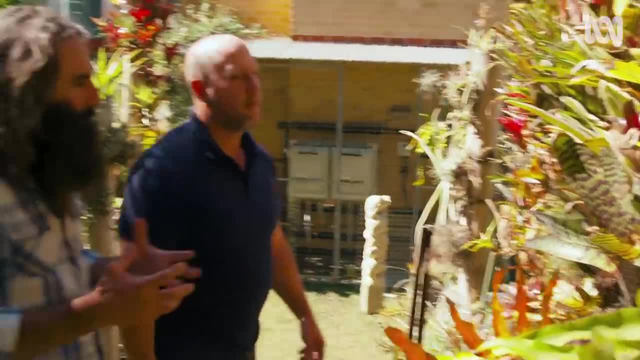 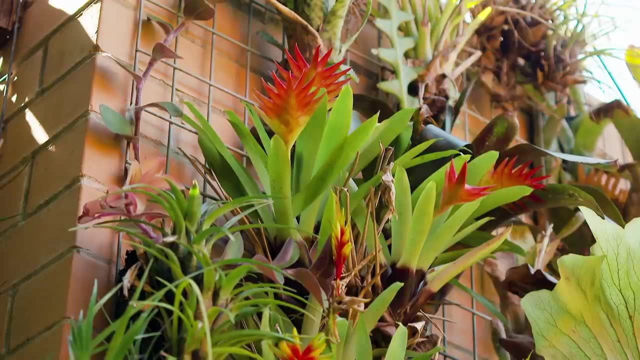 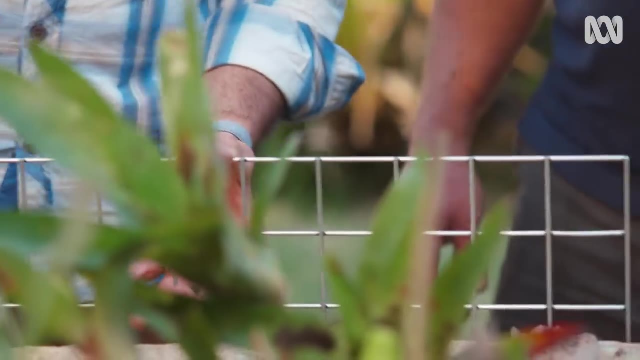 and then you hang it onto that wire mesh. Can we have a go at making one of those? Certainly So. this mesh is really the frame you're going to hang it all off. Yes, I mean, I suppose you could use steel reinforcing. 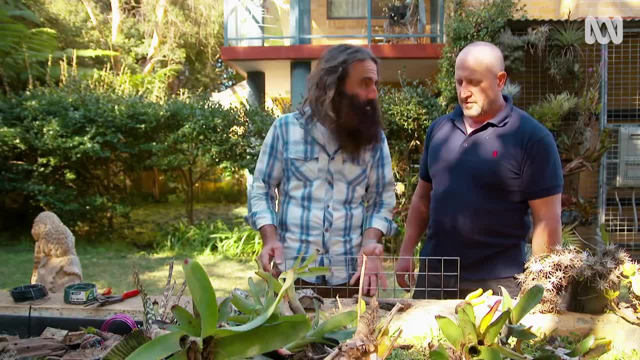 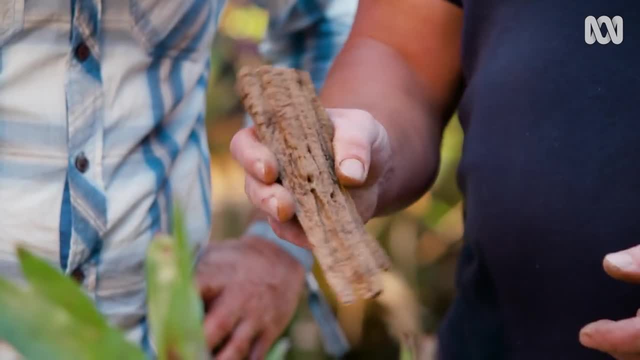 you could use an old gate. you can use old fencing. There's plenty of options. there isn't there. There's plenty of options. that's right. So what we start off with is getting a natural board or timber, or even a piece of plywood. 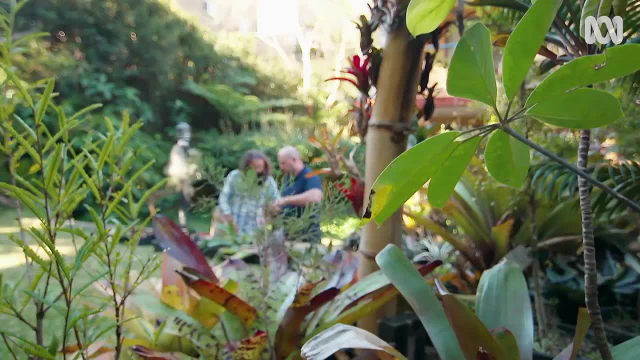 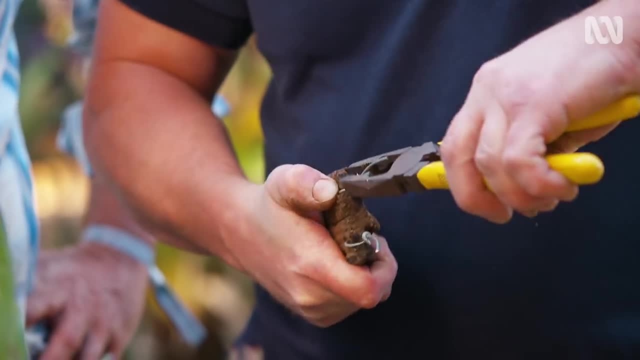 and then I'd get some wire to make some hooks first, And I'll just fold that over And from there twist it on a few times to make it strong, And then you just hook it over, Try and get it about the same height so it sits square. 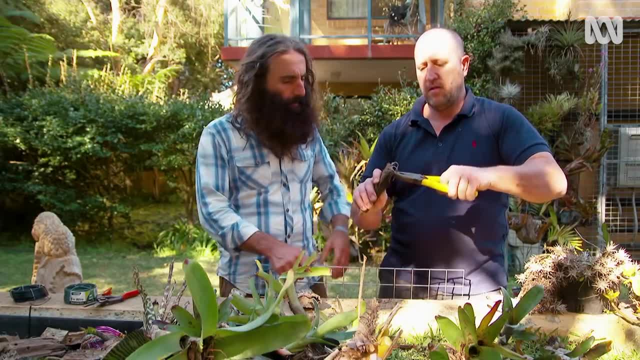 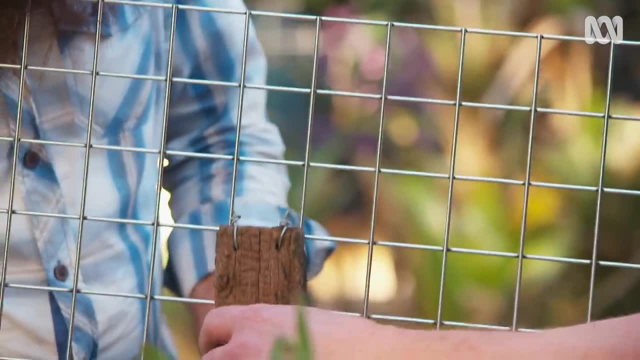 So there's an example. It doesn't have to be too neat because it's just designed to hook on. Oh, Yeah, that's not bad, That's fine. Yeah, that's great. The next step is to attach the plant. yeah, 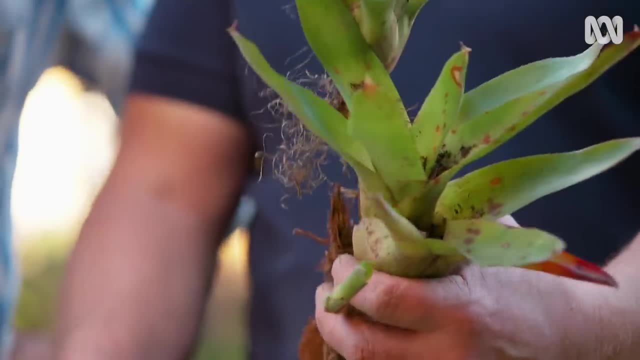 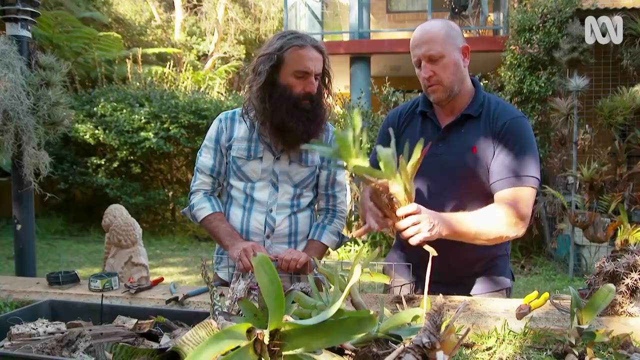 Yes, it is So. here's an example of one here. And you've just pre-drilled some random holes in there, roughly apart. That's right, To enable you to clasp. That's right. All right, that's on there. 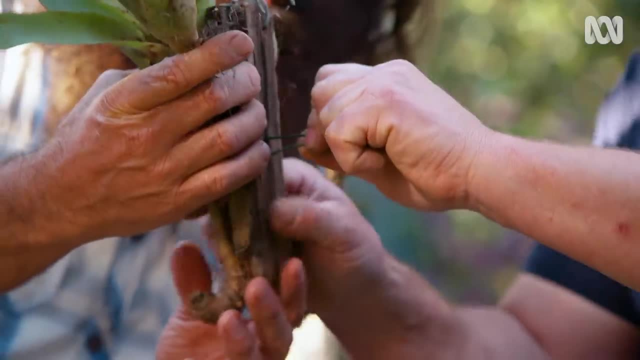 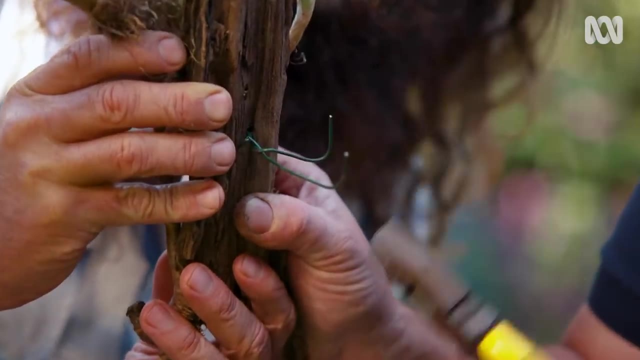 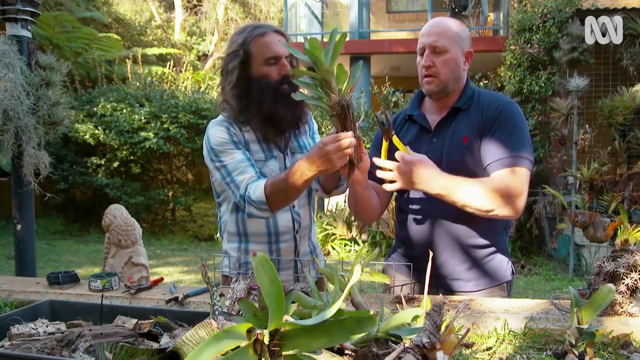 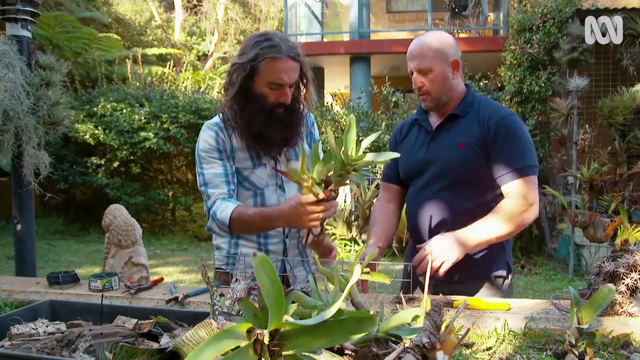 Just need to keep the pressure on to attach it. Some are easier than others, obviously. From there I cut the wire off And hold that down. Yeah, that's nice and solid, And look at that, Let's give it a test run.